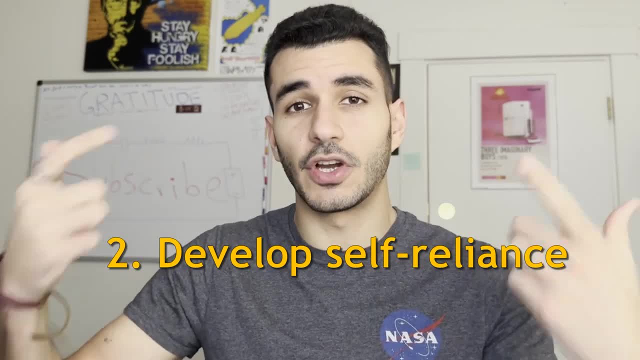 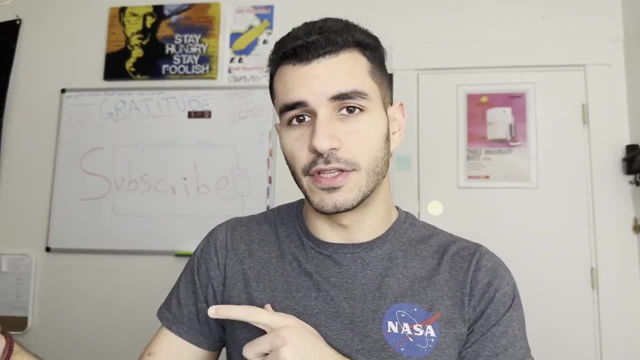 hold your hand. You have to really learn to become independent and be self-starting. And what I mean by that is: no one's going to come and tell you, hey, go apply for this. Or hey, there's this opportunity here. Or hey, there's this professor that's doing that. No one's going to present you. 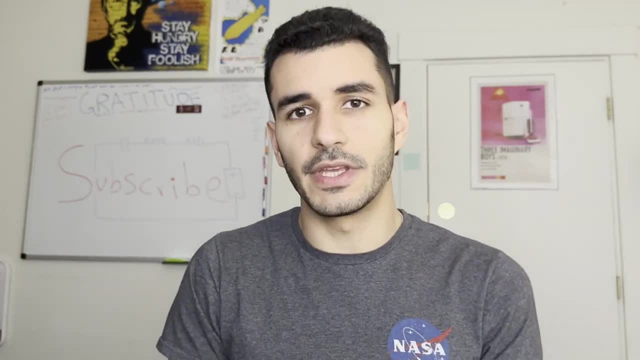 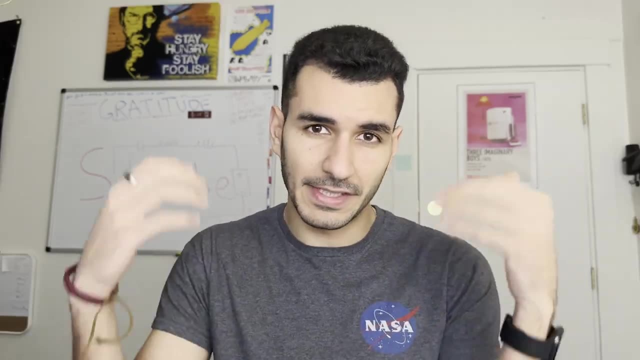 with these things. Sure, you might see flyers, some people might introduce you some things, but you're going to. it's going to be entirely up to you to go ahead and talk to people, join projects, talk to professors, do all these things. You have to learn the skill. 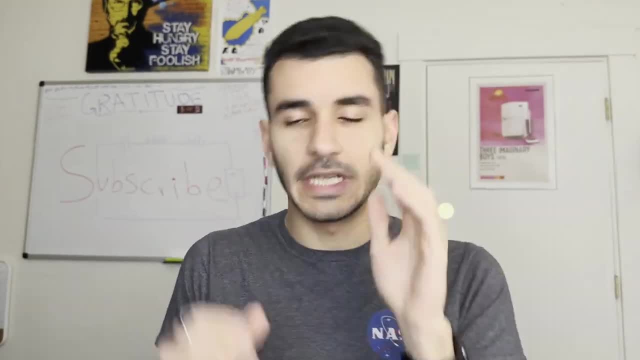 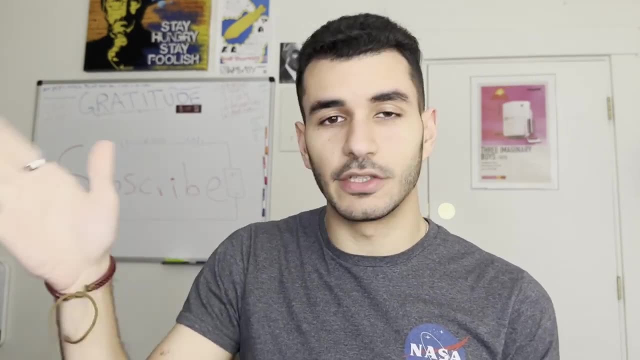 or the character trait of being self-motivated and self-starter, And I see this everywhere, not just in engineering. In any area that I observe the people who are absolutely crushing it. no one's telling them what to do. They're constantly going out and doing stuff themselves. 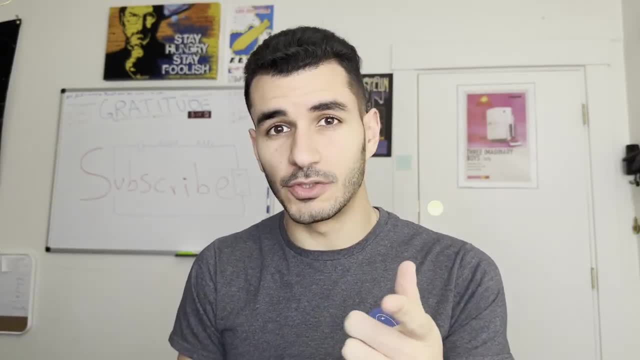 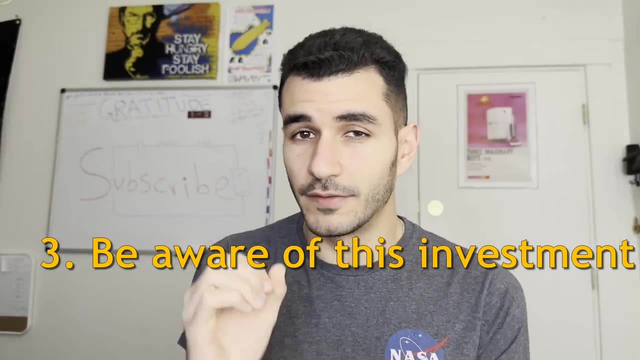 And now, they're not born that way. That's a skill or a habit that they develop, and you can develop it as well. So I would strongly urge you to develop it, Become a self-starter and just go do stuff. Third piece of advice is I want you to understand the opportunity cost of not just the money you're. 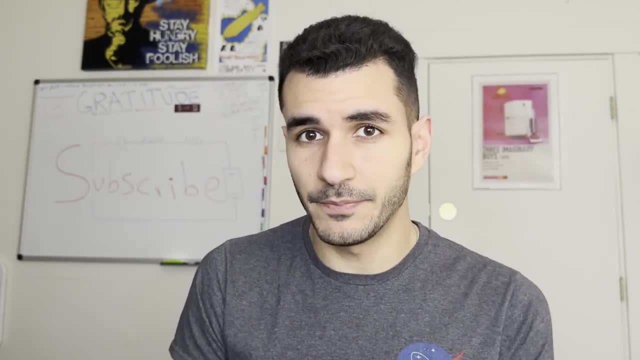 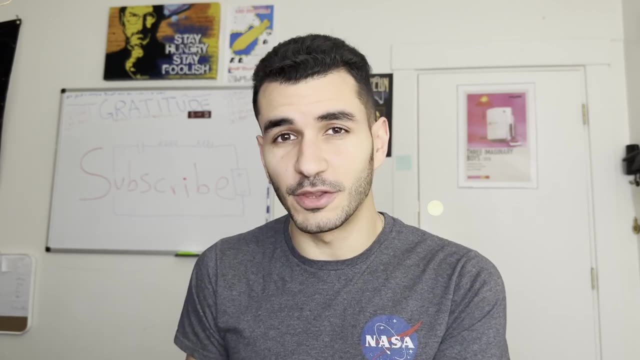 paying for college, but the time If you're going to spend four or five years in a program, those are four or five years you could be spending doing So. you better make the most out of those four or five years in college and you better make the 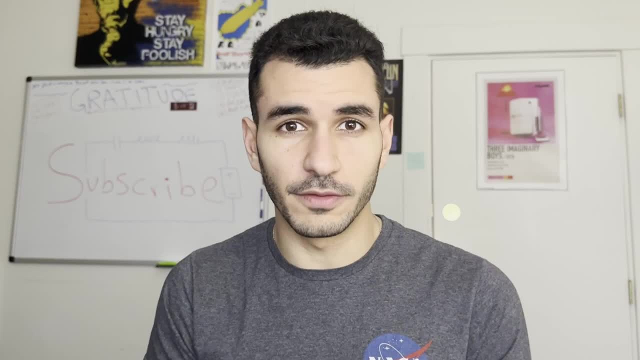 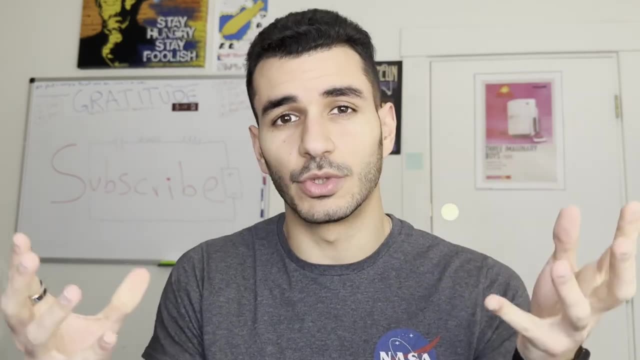 most out of paying all that money for college. Now, one thing you've done which is wonderful, is study a major like engineering, which will have a financial return on investment and also will give you ways to think and approach the world and see the world. So it'll have a time. 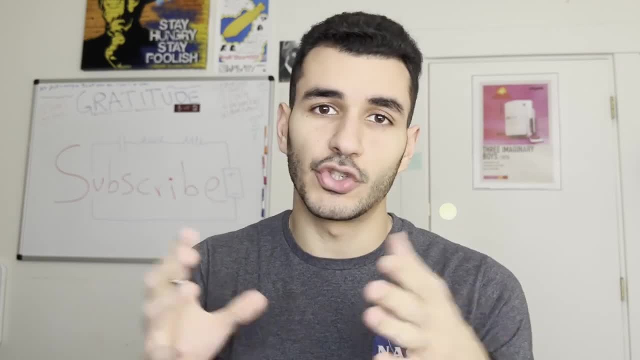 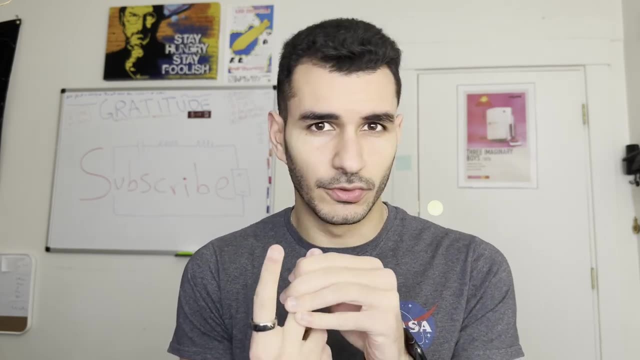 investment on your time as well, but it will again entirely depend on how you actually approach it. There's two students that can graduate with an electrical engineering degree. One guy has really learned the classes, asked questions, joined clubs, joined projects. 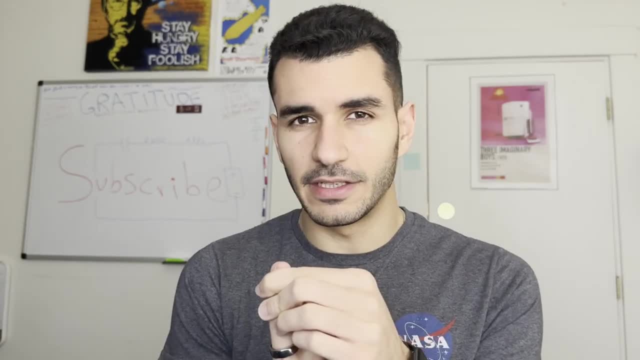 and worked on things hands-on, done internships, And there's a lot of people who have done that and they're going to have a lot of time just kind of cruise by and did absolutely nothing. Both of these people will end up with. 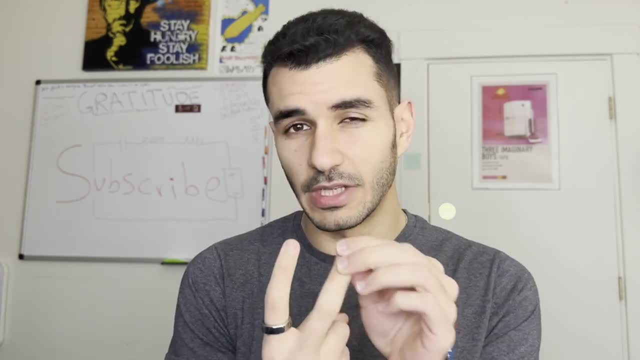 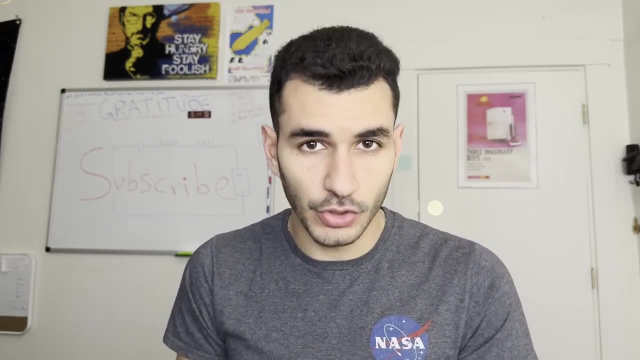 a degree, but one of them will be a lot richer in experience and will succeed later on in life than the other person, So why don't you be this guy? Lesson number four is on a college campus, especially if you're going in person quite often, and you should go in person quite often if you. 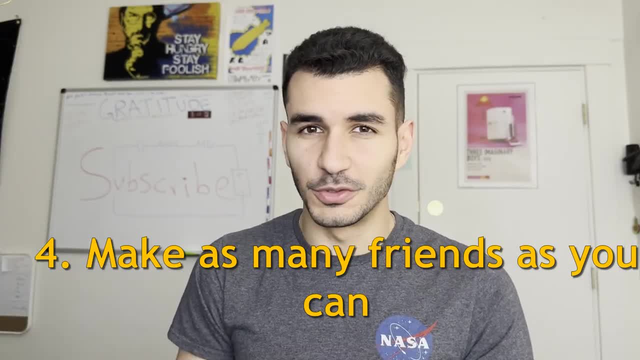 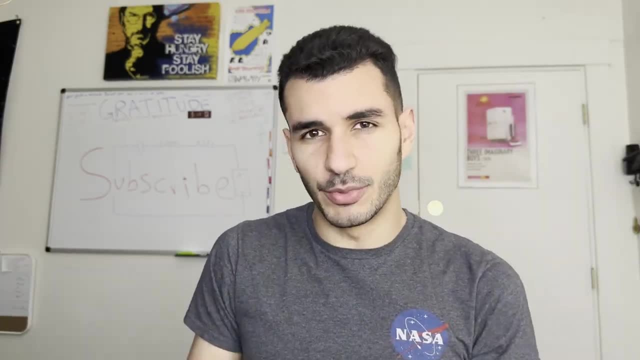 get the chance. your main goal really is to make friends. It's not really to study or get good grades or whatnot- And sure you want to have in the back of your mind that you want to figure out what to do with your life, but the main goal really is to meet people and bump into people. 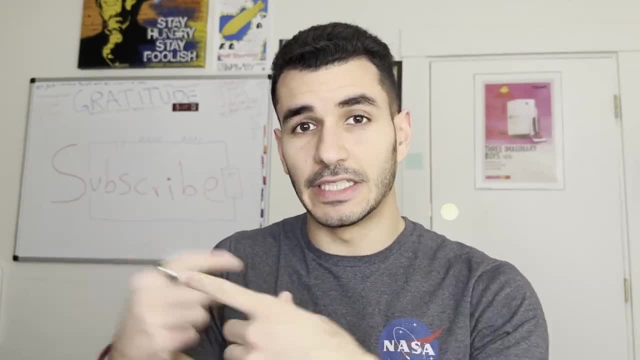 and see what the other people are doing and tell them, hey, this is what I'm doing, and ask what they're doing. and then stop and think and ask, okay, is this what I want, Is this not what I want? And I say this because, from experience, most of the 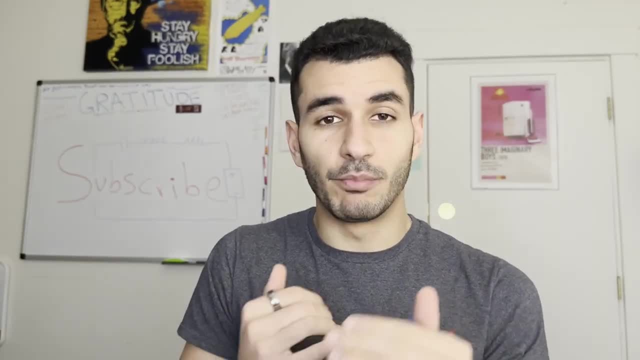 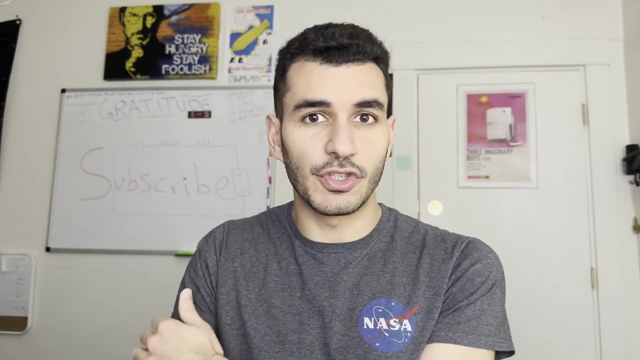 things I learned in college, especially freshman, sophomore year, were from bumping into people who were doing something And I would think, oh wow, this actually seems interesting, Should I be doing that? And then I go and ask them questions about it, And then I assess, and then I joined their 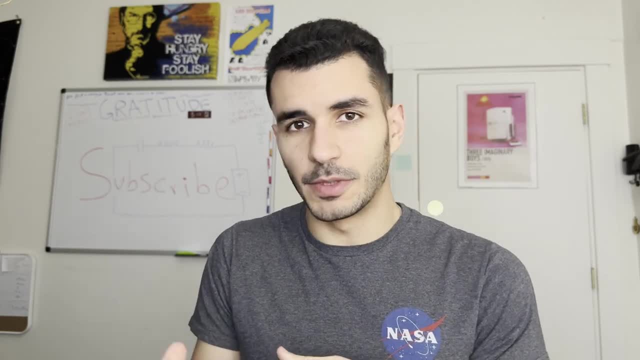 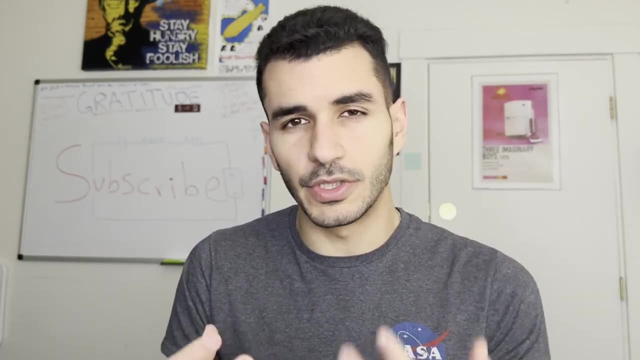 project or club or whatever. Now you can develop the skill of approaching people or whatnot. There's tons of videos and online content on that. If you're somebody who's like, let's say, more introverted and whether you get anxiety around people or whatnot, you can work on these things, But it's 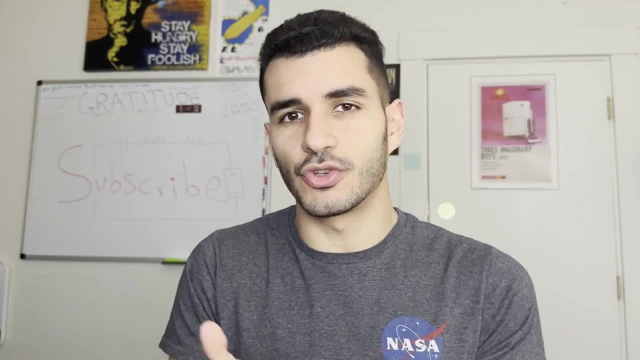 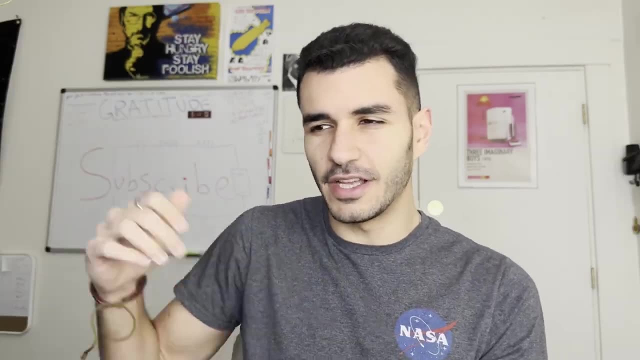 very important that you go approach people, And one easy way to do it is to just join clubs or join projects or join events where people are expected to talk to each other about a professional topic, And that kind of already breaks the ice. That's far easier than just randomly approaching. 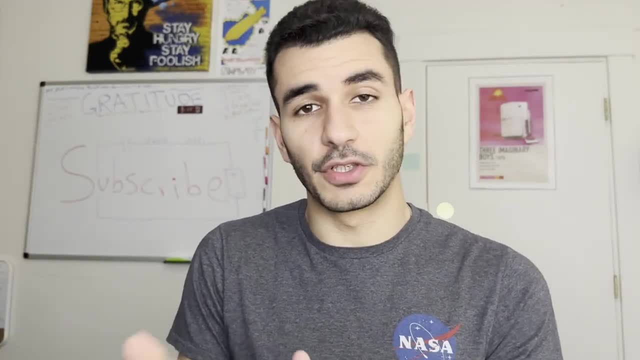 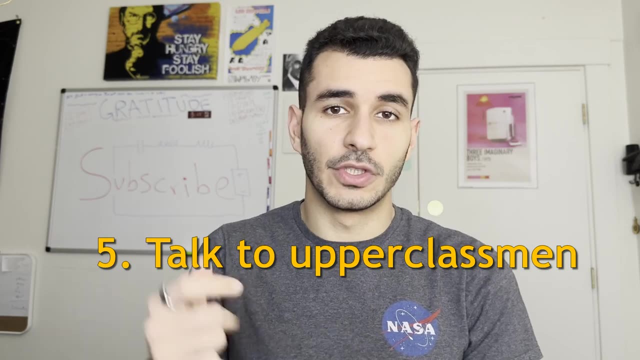 people on campus, But ideally you want to talk to as many people as possible, so you actually figure out what you want. which brings me to the fifth piece of advice is that you want to talk to upperclassmen, So don't spend all your time hanging out with freshmen. Go hang out with 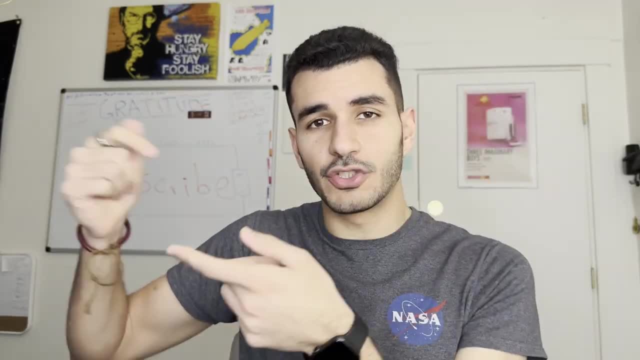 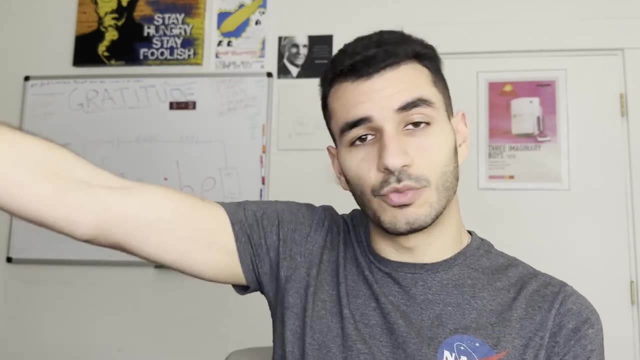 sophomores, juniors, seniors- and see what they're doing And think about it. you're going to eventually be in their shoes. So why not go to these upperclassmen and ask them questions and see what they're doing, And that will help you get insight on what will happen down the road In 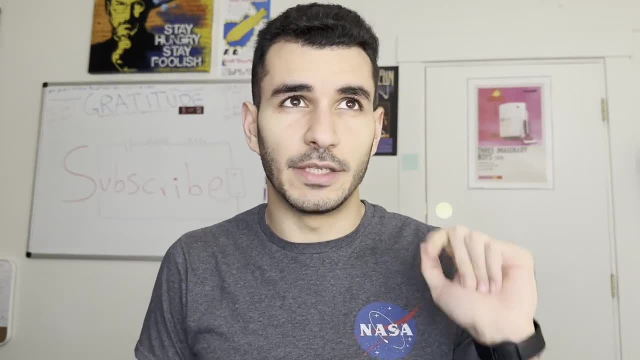 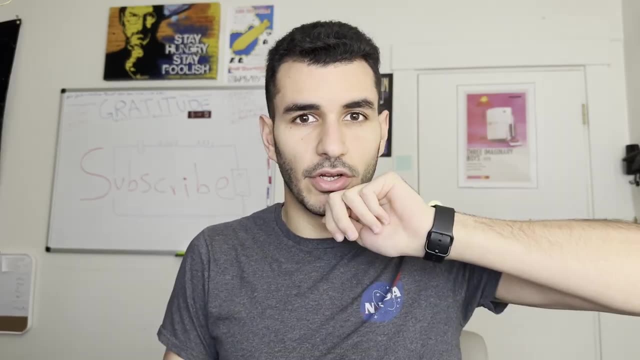 fact, one of the reasons I switched to electrical engineering is when I was a sophomore I met a group of juniors who were in electrical engineering And I took a look at what they were doing And I envisioned myself doing what they're doing down the line And I thought, oh, that's actually really. 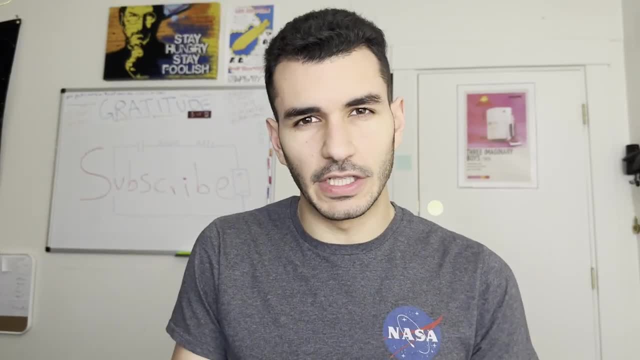 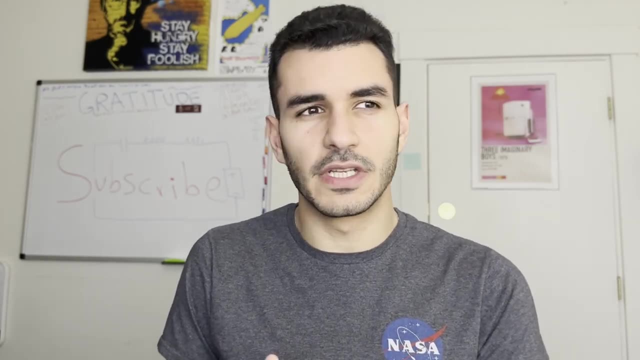 cool. I probably should be working on that And that's how I hit it off. Also, you'll figure out, not so much focus on school- Some people will be like focused on actually getting things done, whatnot, But generally, like junior seniors are like thinking about that next stage, which is 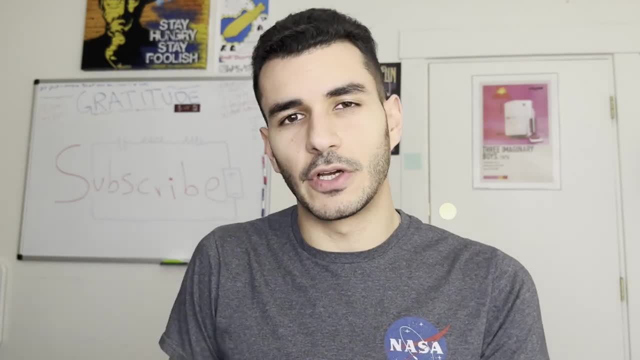 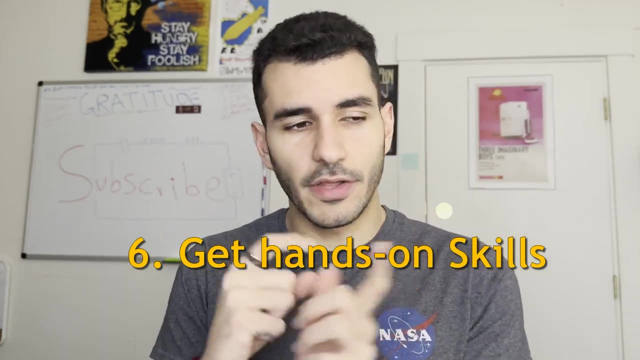 job, graduation, grad school, whatnot. So these are really helpful people to talk to if you're trying to consider what to do for a career. Sixth piece of advice is: you want to get as much hands on experience as possible. And again, nothing against the classes you're going to go to your. 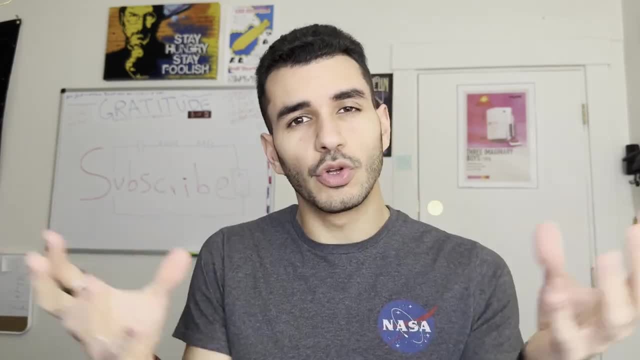 classes and you're going to learn, you're going to ask questions and whatnot And that's gonna be cool, But a lot of that is going to be theoretical knowledge. you really want to get as much hands on and like learn by doing as possible, And that's what I'm trying to do, So I'm trying to get as much. 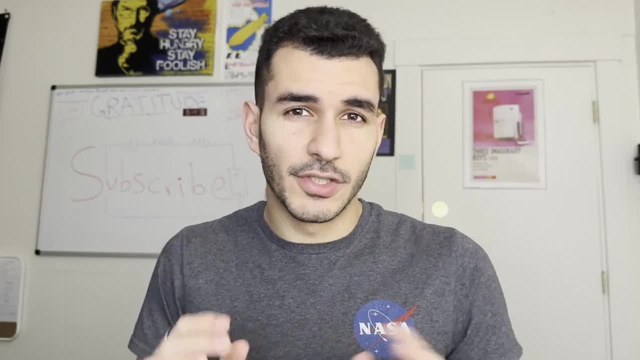 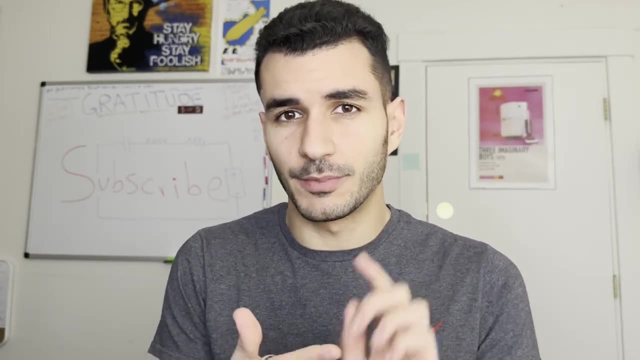 as possible. And seven is you want to be able to secure a summer opportunity, So summertime is usually like really good chance to go get hands on learning or go get experience, whether you apply for an internship or you apply for some type of project, or even if you go back home and work on.